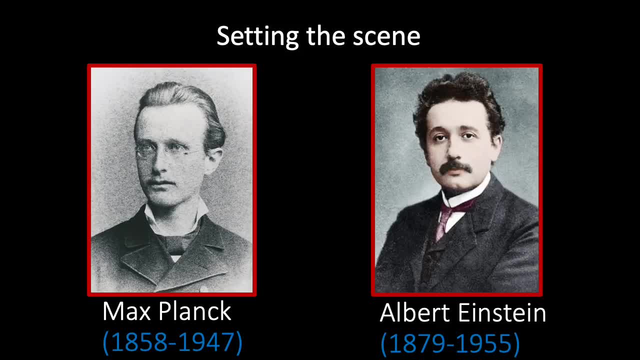 had been based on the idea that light was in fact a stream of particles called photons, rather than a continuously varying wave. These ideas had been based on the pioneering work of Max Planck in 1900, who was able to explain the radiation properties of hot objects by assuming 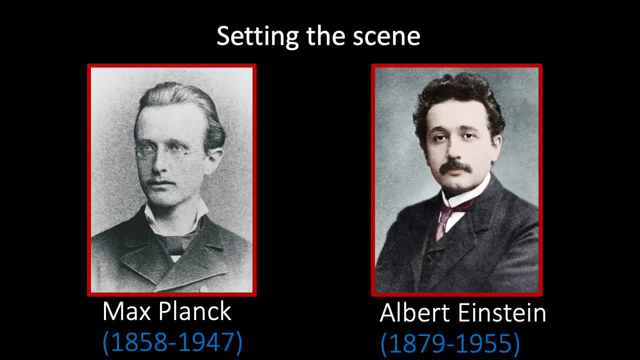 that energy is only ever transferred in discrete chunks or quanta, rather than in the continuous fashion predicted by classical physics. Despite the success of Einstein's photon model explaining the photoelectric effect, many physicists were still reluctant to adopt this new, radical vision of light. 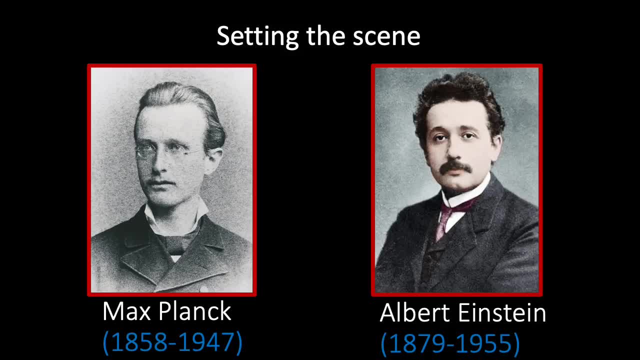 After all, apart from the photoelectric effect, electromagnetism was a remarkably successful theory capable of explaining an incredibly broad range of observations of the natural world. In order for the physics community to take the idea of photons seriously, physicists needed to find another example like the photoelectric effect. 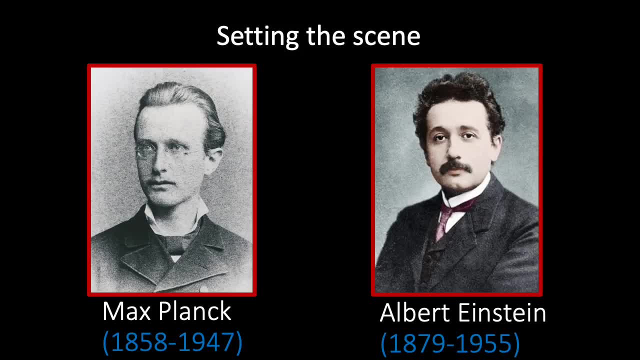 that could be used to explain the idea of photons. The idea of photons was a very important part of the physics community and it was a very important part of the physics community. It was a very important part of the physics community. It could only be explained by the photon model of light and this would require a top-rank. 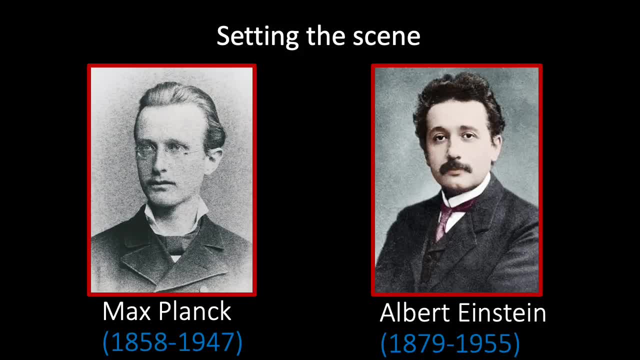 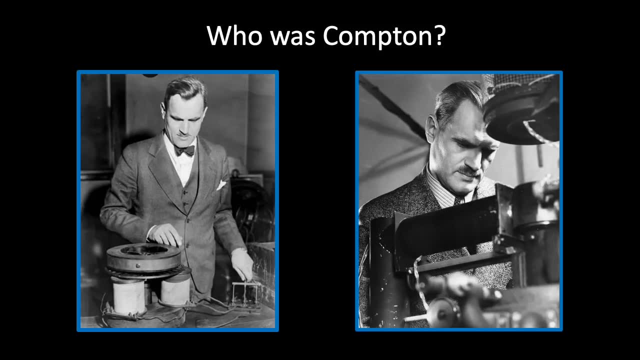 experimental physicist with an appreciation for the work of Einstein and Planck. His name was Arthur Compton. In 1919, after completing his PhD at Princeton, Compton was awarded one of the first two National Research Council fellowships that allowed him to study at the Cavendish Laboratory in Cambridge, England. 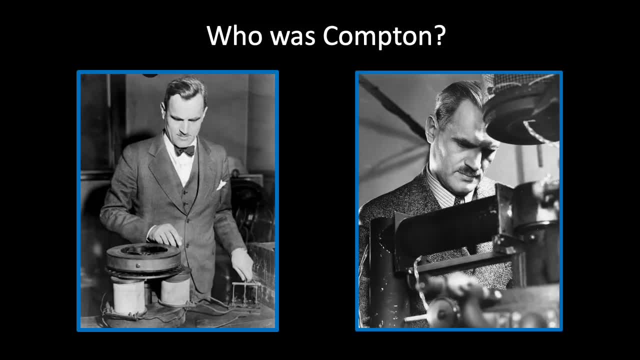 It was here that Compton studied the scattering and absorption of gamma rays under the guidance of George Thompson. George Thompson was the first to study gamma rays under the guidance of George Thompson. JJ Thompson's son Returning to the United States, Compton was appointed professor of physics at the 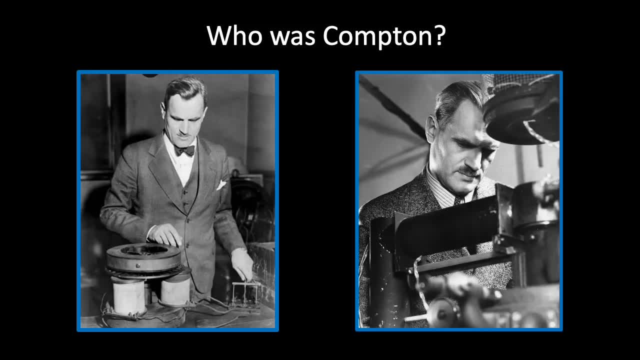 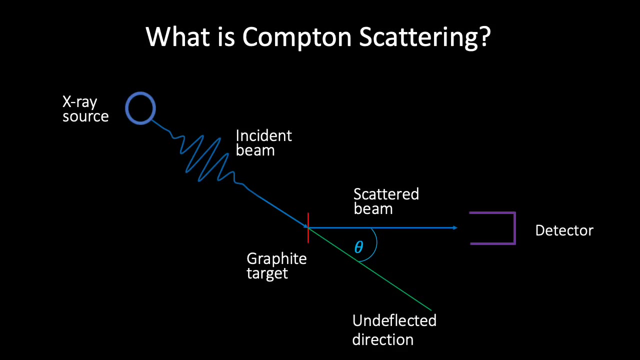 Washington University in St Louis, and two years later, in 1922, he produced his groundbreaking work on X-ray scattering that would once and for all confirm the photon theory of light. Compton's experiment involved directing a beam of X-rays of sharply defined wavelength. 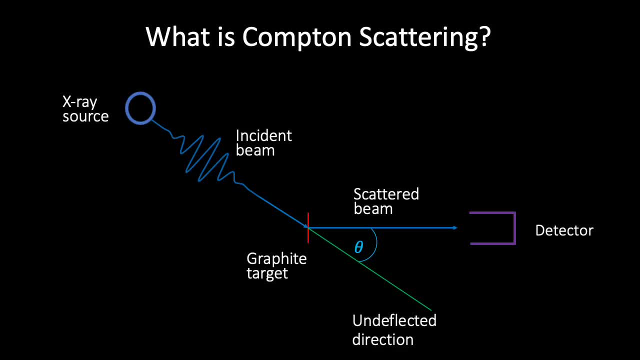 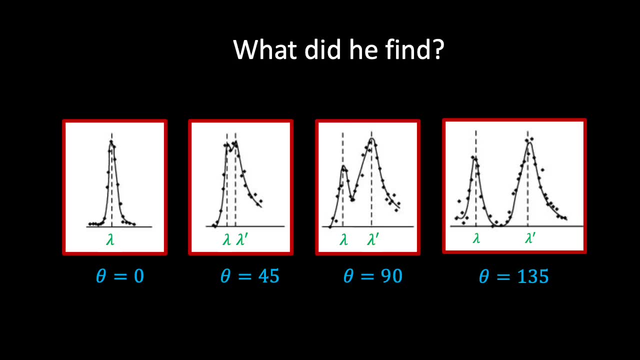 onto a graphite target For various angles of scattering. he measured the intensity of the scattered X-ray scattering and then measured the intensity of the scattered X-ray scattering. Compton discovered that, although the incident beam consisted of X-rays of a single wavelength, 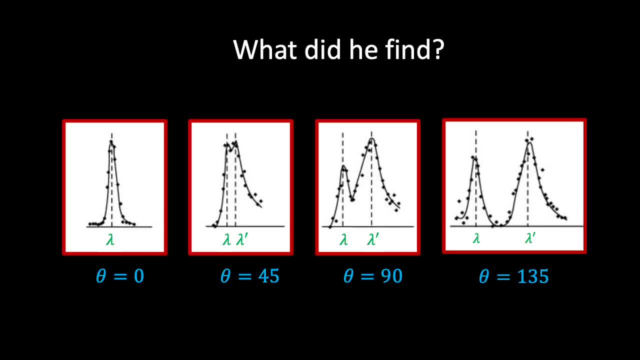 lambda. the scattered X-rays have intensity peaks at two distinct wavelengths: lambda and lambda prime. One of these peaks is just the same as the incident wavelength, lambda, whereas the other is larger by an amount delta lambda equals lambda prime minus lambda. We can also see from the data: 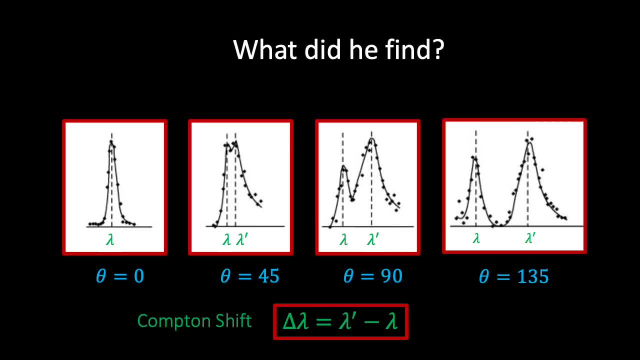 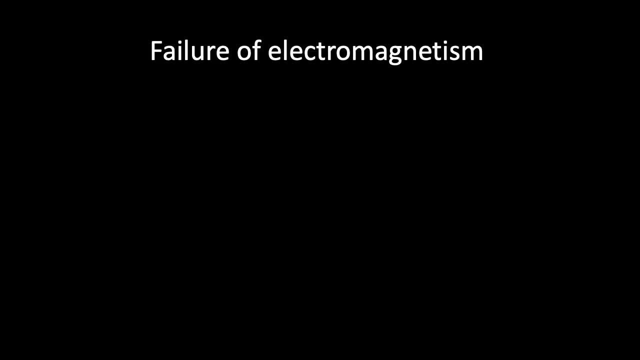 that this beam of X-ray scattering is a function of the wavelength. So what did he find? Compton discovered that the Compton shift in wavelength varies with the angle at which the scattered X-rays are observed. So how can we understand this experimental result? According to electromagnetic 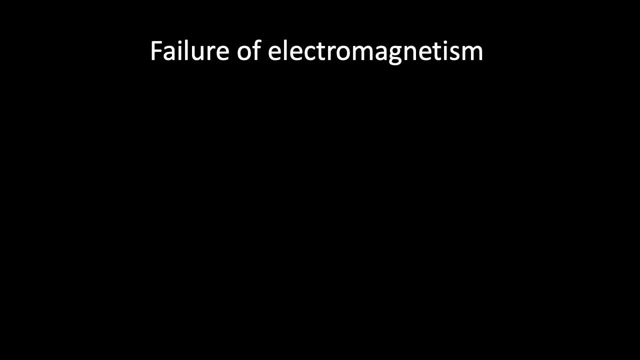 theory, the incoming X-rays should be regarded as electromagnetic waves with a frequency corresponding to the frequency of oscillation of the electric field component of the wave. The incident X-rays would cause the free electrons inside the graphite target to start oscillating with the same frequency. 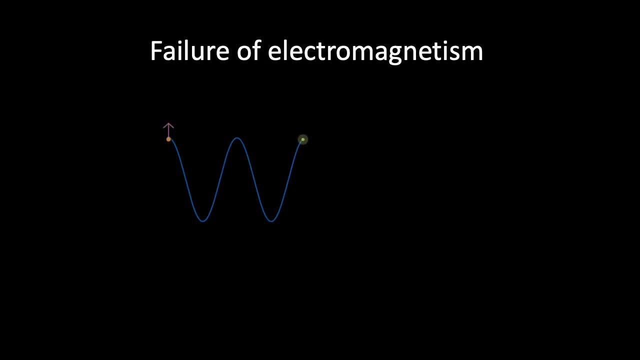 as the incident wave, And this would then cause the oscillating electrons to emit electromagnetic radiation with the same frequency. If the frequency of the emitted radiation is the same as the incident radiation, then so too is the wavelength, and therefore we see that classical electromagnetic 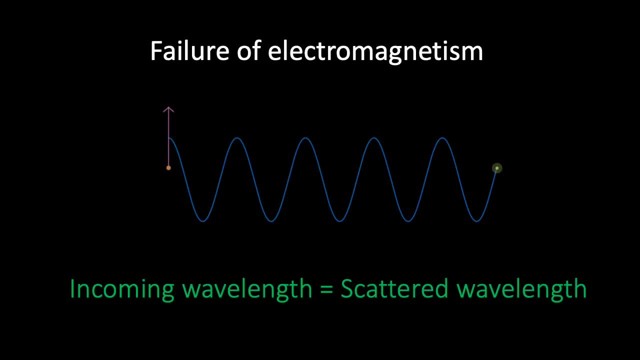 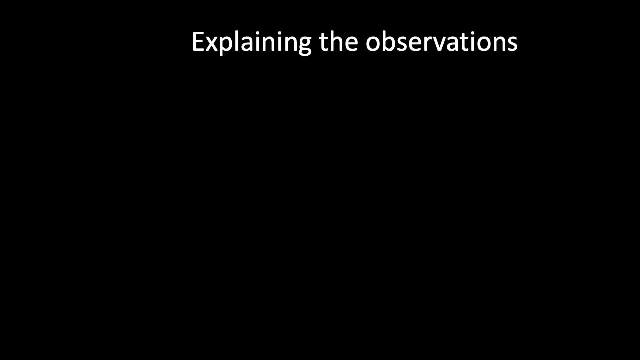 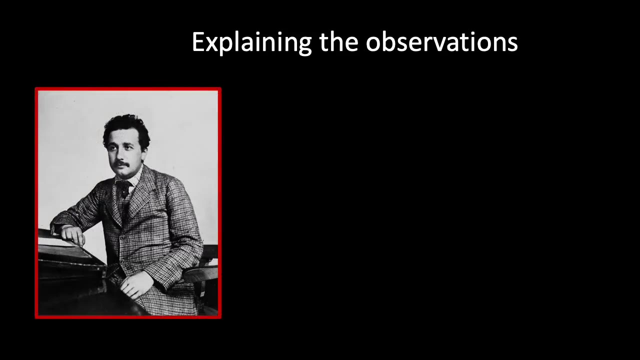 theory predicts that there should be no Compton shift in wavelength. However, as we've seen, this was not what was observed. So how does one interpret this result? The key to Compton explaining his experimental results was to use the photon model of light introduced by 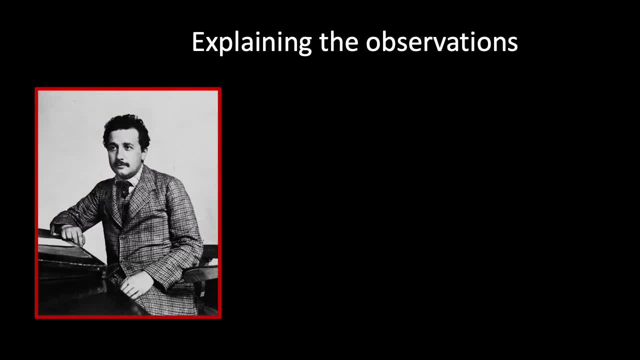 Einstein in 1905.. Compton assumed that the incoming X-ray beam consisted of a stream of photons, each with energy HF, and that these photons collided with free electrons in the graphite in a one-to-one collision, much like two colliding billiard balls. According. 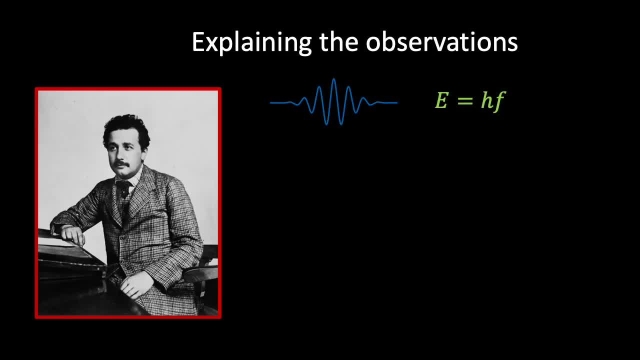 to this view. it is the individual photons that are scattered due to their collision with the free electrons inside the graphite. Since the incident, photons were scattered. the individual photons were scattered. The individual photons were scattered and the photon transfers some of its energy to the electron that it collides with, the scattered. 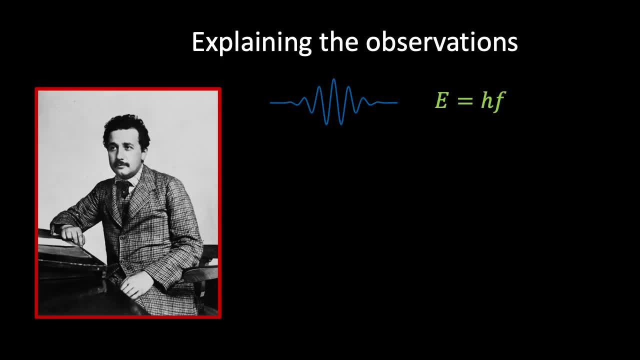 photon will have a lower energy than the incident photon. Now we know that the energy of a photon is proportional to its frequency, and because C equals F lambda, we can see that the energy of a photon is inversely proportional to the wavelength. and so if the energy of 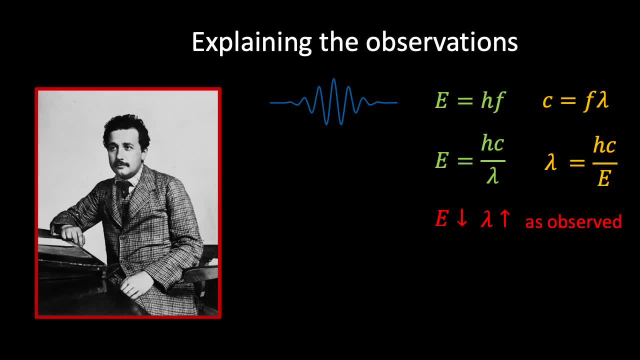 the photon reduces, then the wavelength will increase, as observed. Now you might be wondering how it is possible that a massless photon could possibly collide with an electron. but it is possible that a massless photon could collide with an electron and transfer momentum. 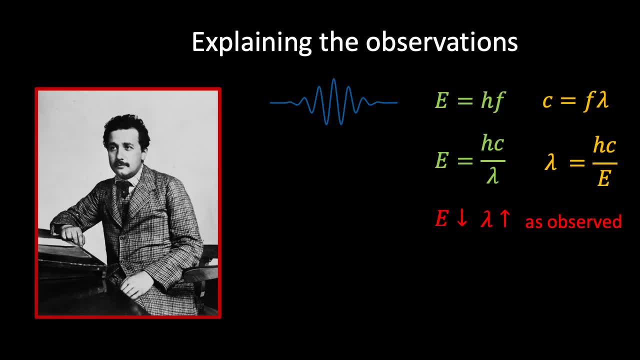 to it, since, according to classical physics, the momentum of an object is equal to the mass, times the velocity. and if the mass is zero, then surely the momentum is also zero. However, according to Einstein's special theory of relativity, the total relativistic 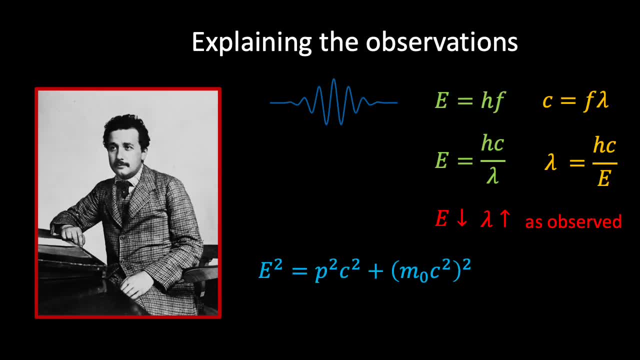 energy of a particle is calculated using the relativistic equation shown below. M0 refers to the rest mass of the object. According to Einstein's theory of relativity, only massless objects are able to travel at the speed of light, and since a photon, by definition, travels at the speed 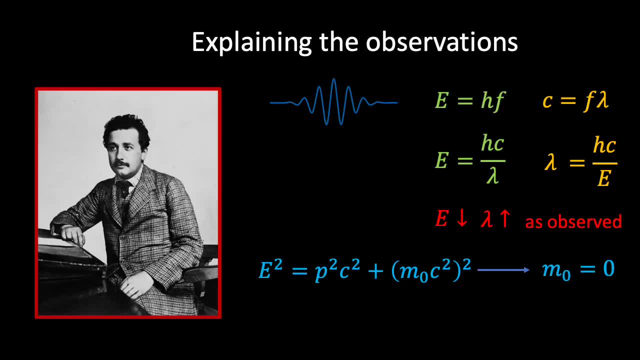 of light, it must be massless and therefore, if we set M0 equals to zero, we see that the momentum is equal to E over C and therefore, if we combine this with the relationship E equals Hc over lambda, we arrive at an expression for the momentum: P equals H over lambda. 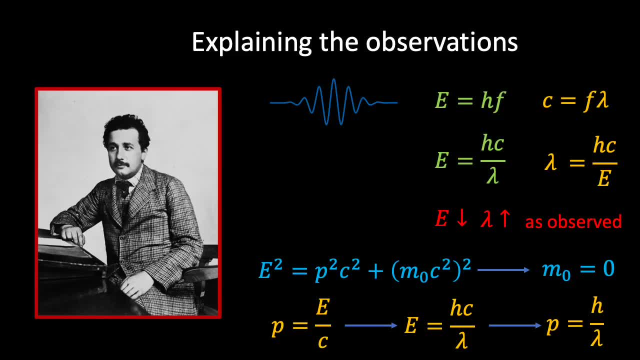 Compton also noticed that the wavelength of the scattered radiation was independent of the material contained within the totality. Compton also noticed that the wavelength of the scattered radiation was independent of the material contained within the totality. This implied that the scattering process did not involve the whole atom. Compton therefore assumed that the scattering was due to collisions between X-ray photons and individual electrons inside the target. 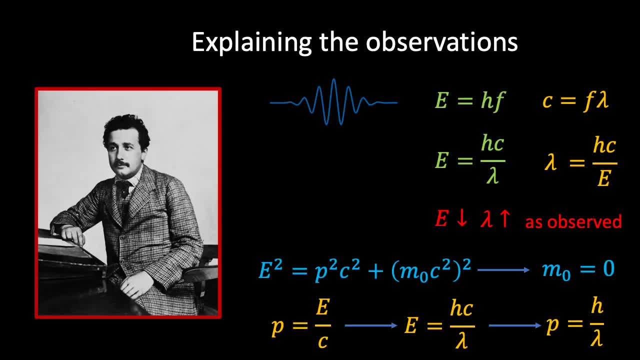 He also assumed that these electrons would behave exactly as if they were completely free, provided that the light quanta which hit them carried sufficiently large amounts of energy. Armed with a way of calculating the momentum of the photon, Compton was able to use the principle of momentum conservation. 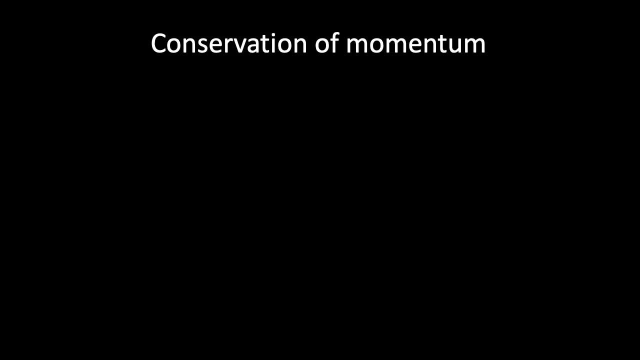 to provide a detailed calculation of the electron-photon interaction and predict the change of wavelength of the scattered photon. Let us now consider this calculation. We begin by introducing an X and Y-axis and locate the electron at rest at the origin. We will assume that the incoming X-ray photon has energy, Ei and initial momentum Pi aligned along the X-axis. 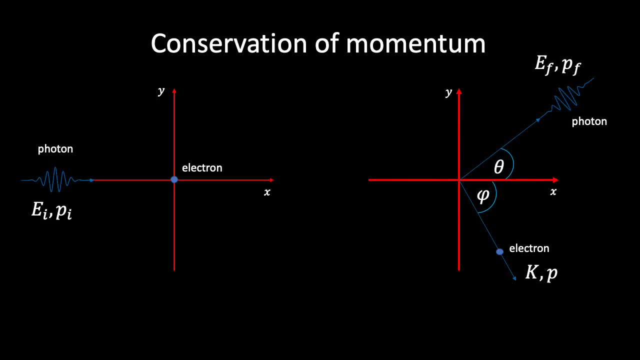